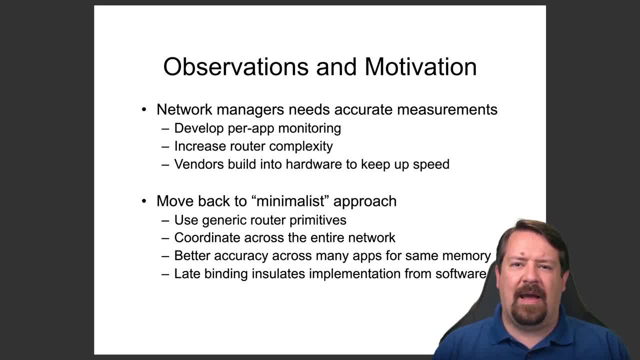 sampled NetFlow And basic NetFlow had scalability issues, And sampled NetFlow didn't meet everyone's needs equally, So there were various things built on top of this, which are what we're calling here per application monitoring, So additional monitoring beyond NetFlow, to answer a particular. 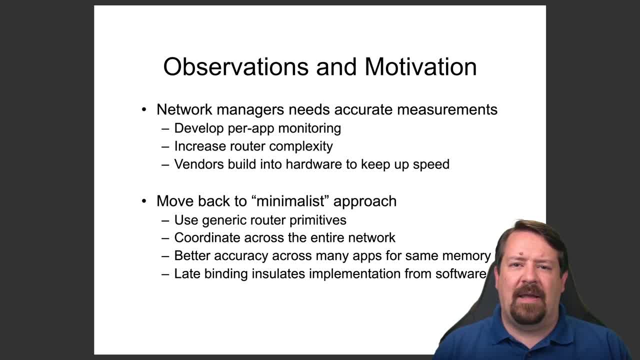 question about the traffic on the network. So the application here is not the application generated by the network. It's not the application generated by the network. It's the application generated by the traffic on the network. It's an application that is providing the network operator a specific 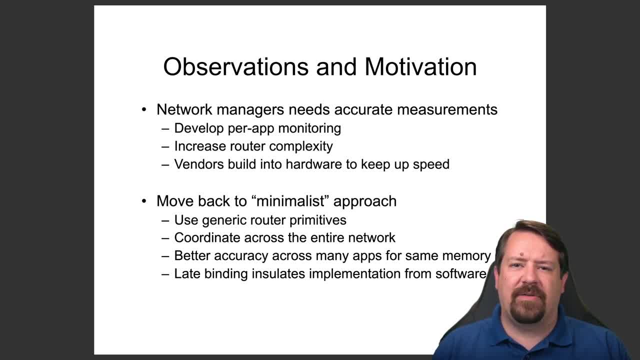 type of information about the network, And so supporting each of these different types of monitoring was increasing the complexity of routers, because it would have to capture metrics in a slightly different way for different applications, And also most of this monitoring had to be done at line speed, So it meant modifying the hardware on the router interfaces. 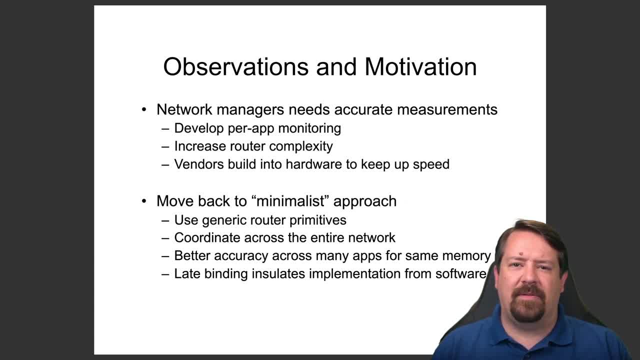 to accomplish it. So the authors are saying that when adding complexity to the hardware, if that complexity could be used with a minimalist approach, using a generic router primitive, it could provide more net benefit than if it was having to deal with each of these individual. 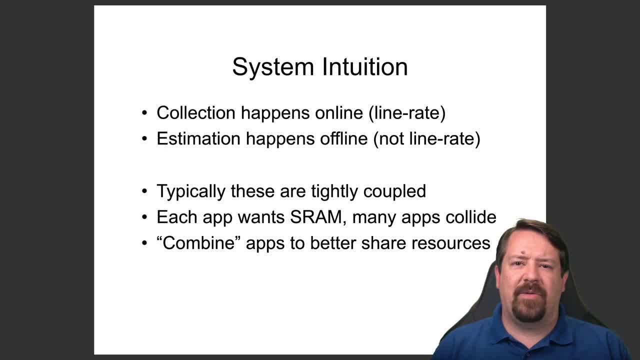 application-specific monitoring tasks. So, as we saw with the NetFlow architecture, we have the collection. that's happening at line rate And then the flow data is shipped off to a collector that does things in the background, so not at line rate. If we look at the hardware of the interfaces, 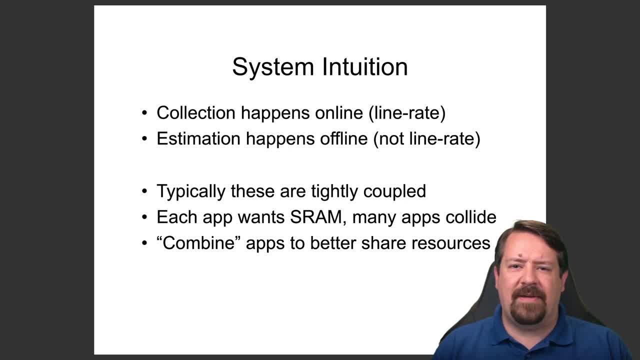 there's a very scarce amount of SRAM, which is the memory that is fast enough to keep up with the interface or events happening at line rate, And if each application needs some of this SRAM, then that's a very scarce resource that is oversubscribed. So the idea here is to make 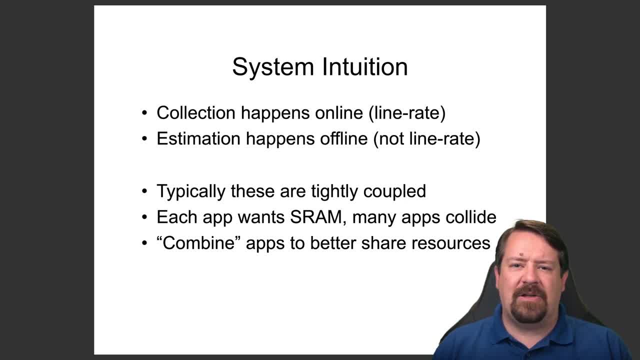 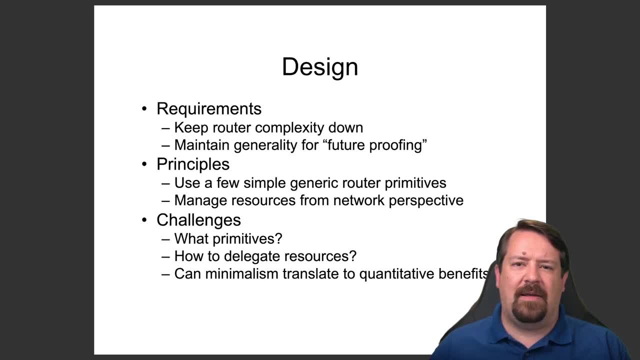 apps share some measurements that the SRAM can perform, rather than each application needing its own piece of the SRAM to do its own measurement. So some of the benefits of this are that it would keep router complexity down And, if done in a really smart way, it could also 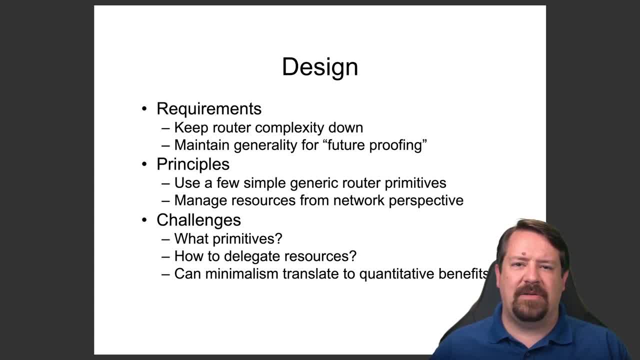 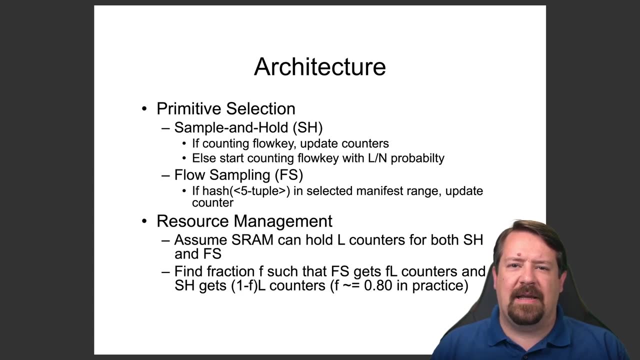 help future-proof the router hardware design. However, this is easier said than done, So the question is what primitives should be tracked that would support multiple applications equally well, And assuming there's multiple primitives, then how should the resources be delegated across those? The authors selected two primitives to look at for this analysis. The first one is called: 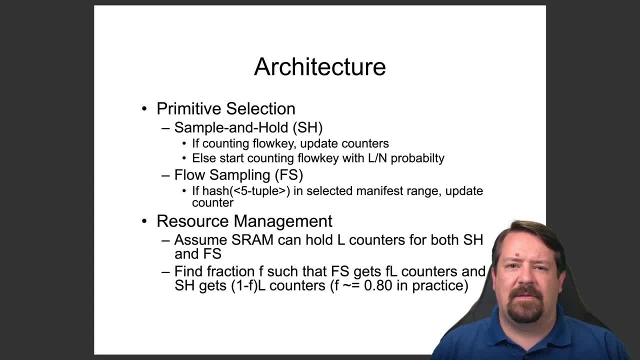 Sample and Hold, or SH for short. So in this case, if the router interface is already tracking a particular flow, it will update the counters for that flow for every time. the interface is tracked For every single packet that matches it. So unlike SampleNetFlow, where it would only get. 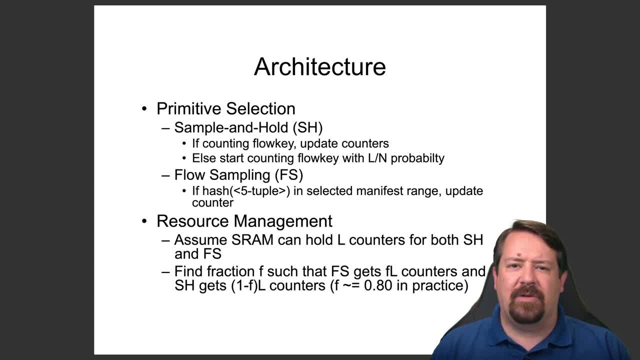 1 in 1000 packets or 1 in 10,000 packets. it's going to track the flow with very high fidelity. However, it won't track every flow If a packet comes in and it's not already tracking that flow. 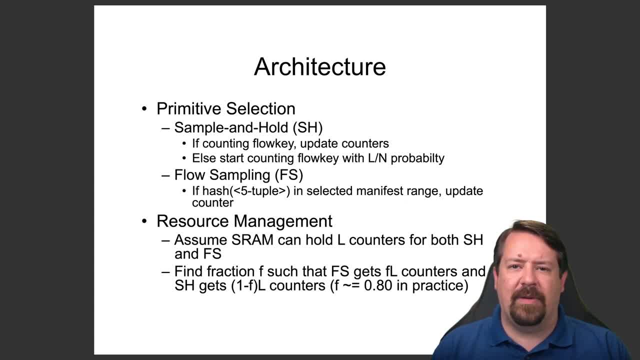 it will only begin tracking the new flow with some probability- L over N in this case. On the other hand, we have flow sampling. So in flow sampling the flow key is hashed And it is only tracked if the hash falls in a selected range. So for those not familiar with 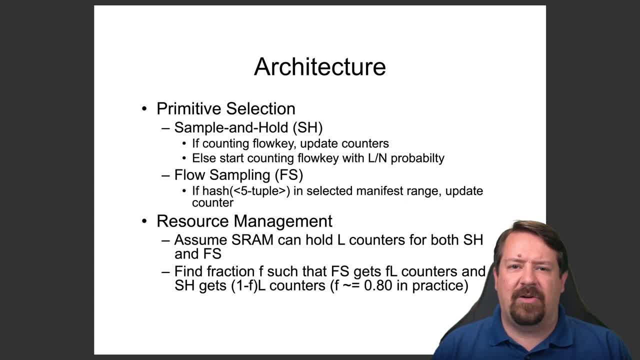 hashing. it's a way of permutating a set of bits in a deterministic manner but at the same time distributing the output uniformly over the range supported by the hash function. So the idea here is to get a uniform sampling of the flows and then track every packet matching those flows. 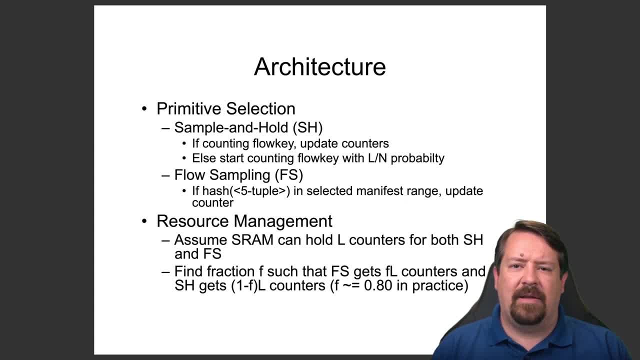 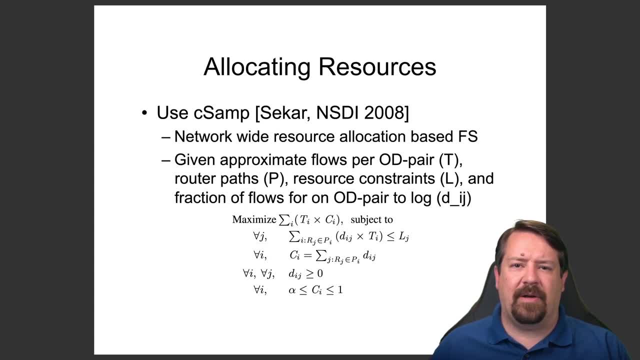 On the resource side, we're assuming that the SRAM can hold L counters, and those have to be shared by the two different primitives. The authors then look at how to allocate resources across the network, And so they're looking at the input- output pairs of the traffic flows and determining how the 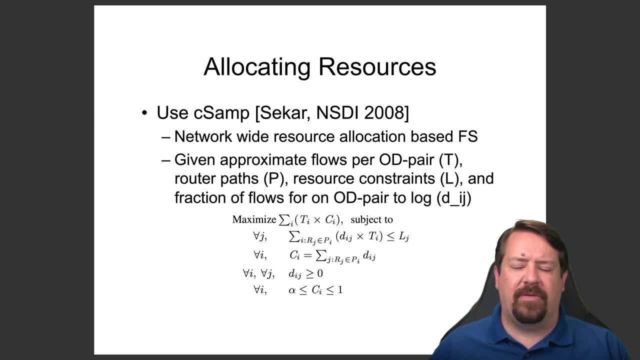 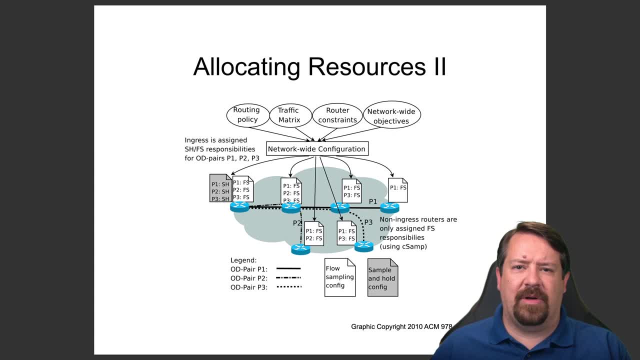 SRAM resources should be divided by these primitives for different routers in the network. And so in this figure we have an ingress router on the left, And we see that the ingress router is running both primitives- sample and hold- as well as flow sampling, But all of the non ingress routers are only running flow sampling. 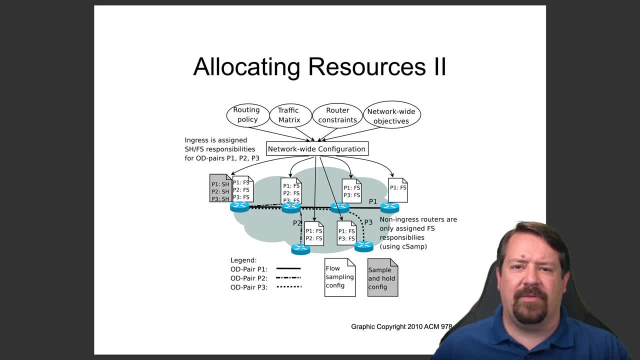 So this is because the hash function used on the flow key is deterministic, So the routers can be configured to track non-overlapping sets of flows, And so it's not redundant for subsequent routers to also run flow sampling. However, sample and hold is a random function, and so it's likely that subsequent routers running 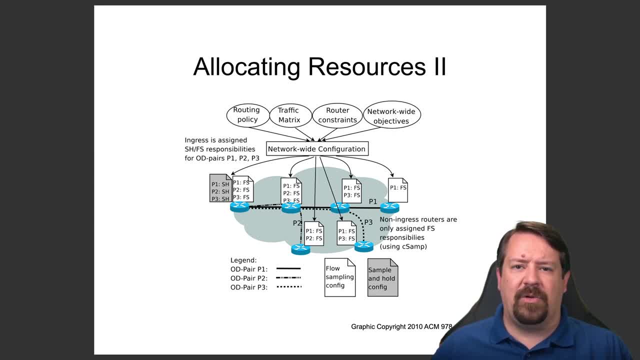 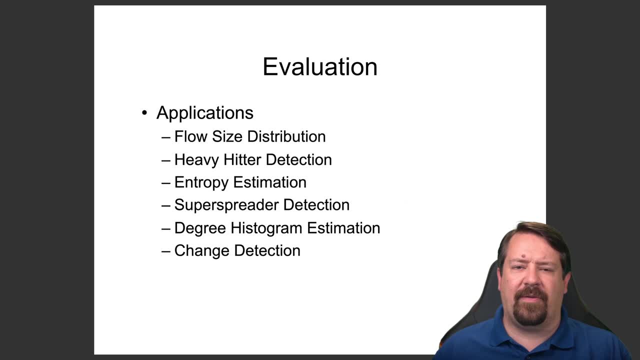 sample and hold on the same traffic would capture redundant information. So, then, the applications that they want to look at, meaning the analyses that they want to perform on this network. traffic collection is a flow size distribution, heavy hitter detection, entropy estimation, superspreader detection. 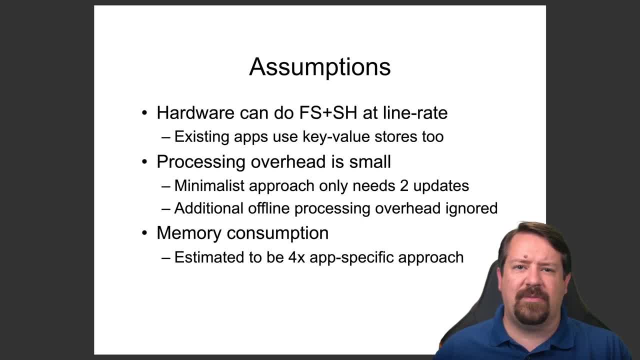 degree, histogram estimation and change detection. The assumptions are that the hardware can do flow sampling and sample and hold at line rate, And this is reasonable given the existing primitives being tracked by the routers. Then there's the assumption that the processing overhead is small, meaning the changes that need 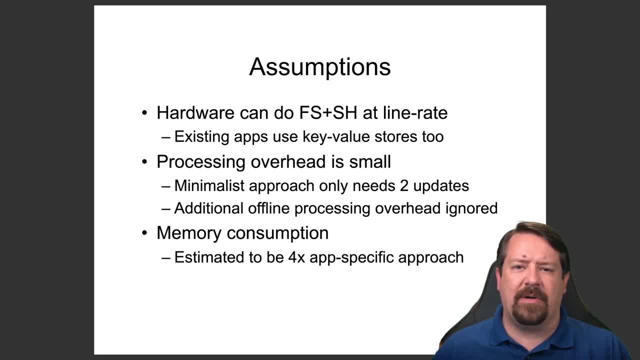 to be made in memory on a per packet basis And there's an estimate about memory consumption. So it's important to recognize for this paper that there's not an actual hardware implementation. These are based on assumptions looking at the capabilities of the hardware, that 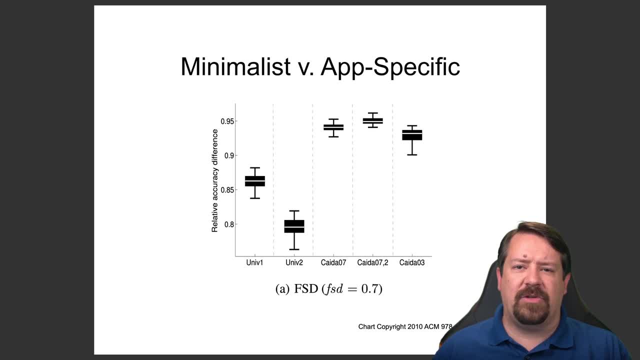 was in use at the time. The authors also used five different traffic sources and found that the results varied somewhat depending on the source of the traffic. So here we're looking at the results for the flow size distribution, meaning that by using the two primitives that they chose, 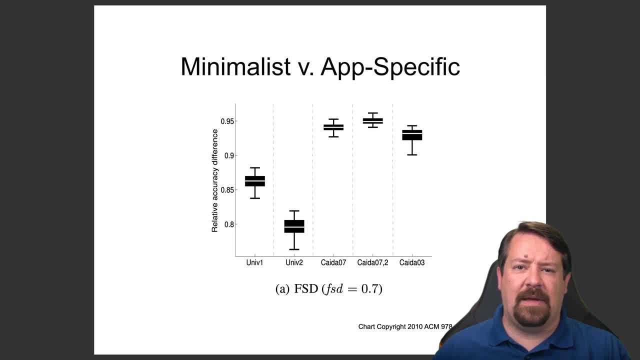 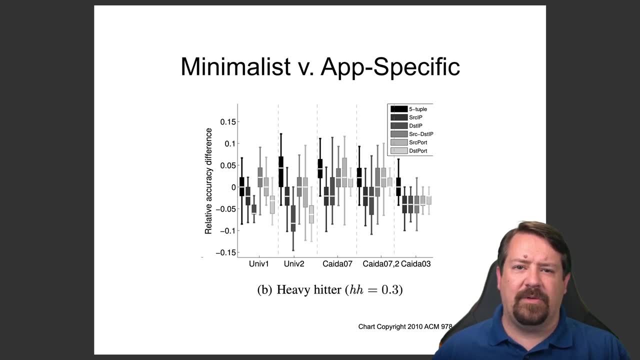 to determine flow size distribution. they're achieving an improvement in accuracy of 80% to 95%. For the heavy hitter application they're seeing an accuracy that is comparable to the original accuracy, some above and some below depending on the source of the traffic. 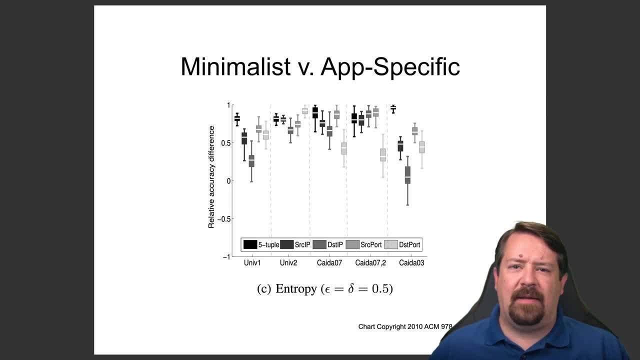 and which particular fields are being tracked. And in the entropy detection they're also seeing a significant performance improvement using the minimalist approach. So we want to note where this gain is coming from Right. Their assumption is that, rather than taking their available SRAM, 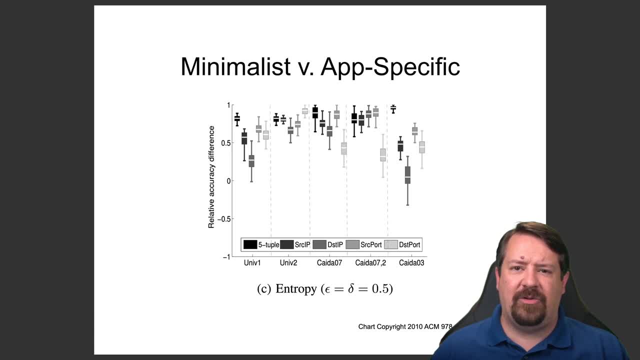 and having to divide it amongst specific applications, so each application only gets a small fraction of that SRAM. they're able to dedicate all of the SRAM to doing sample and hold and or flow sampling and then take the results of those two and compute these other metrics. 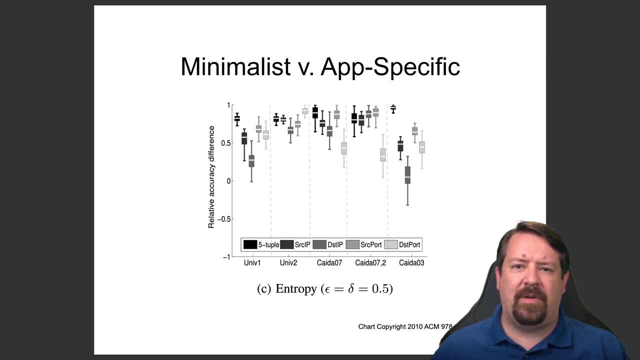 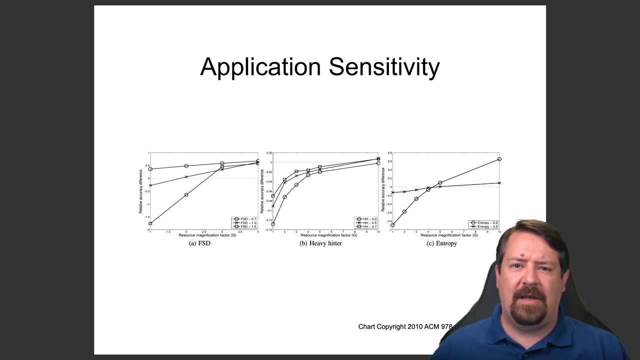 So the ability to see an improvement in a particular application depends on whether the primitives that they chose are suitable for computing that application. So here we see that, depending on how efficiently they're able to use the resources, their result could be significantly worse than the application. 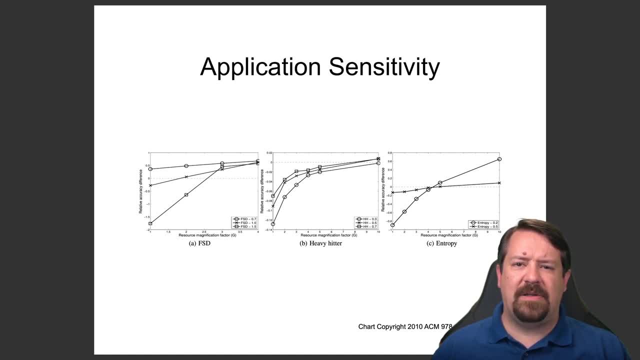 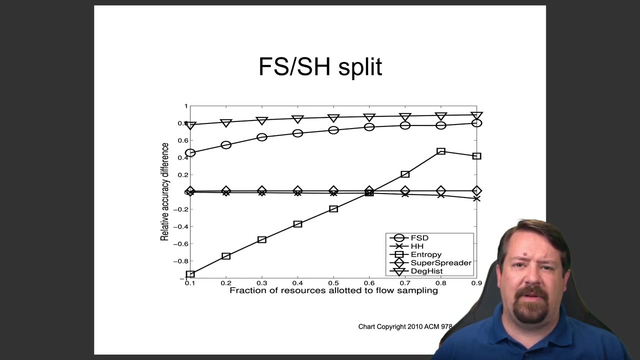 specific method or significantly better, And this speaks to the importance of the assumptions that they're making here and how accurate they are in terms of the amount of resources needed to compute, sample and hold or flow sampling. They then look at the result of splitting their resources between flow sampling versus sample and hold.